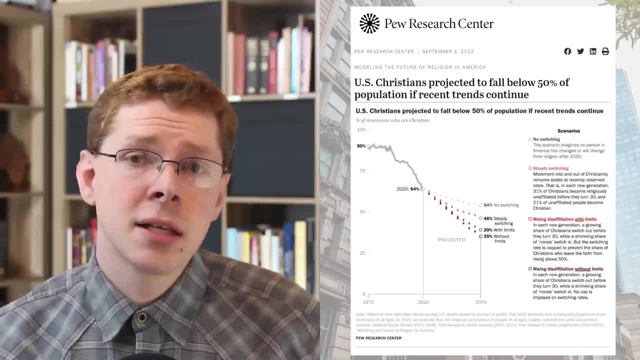 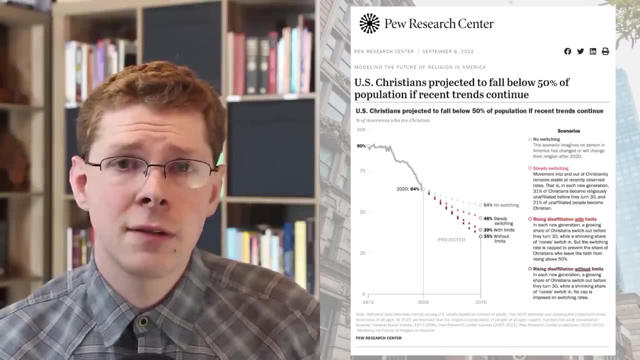 or even a bar. The number of professing Christians in America is declining. In September 2022, Pew Research Center modeled that by 2070, Christianity will almost certainly be the religion of less than 50% of the US population. In the UK, where a 2021 census revealed that Christianity is already a minority, 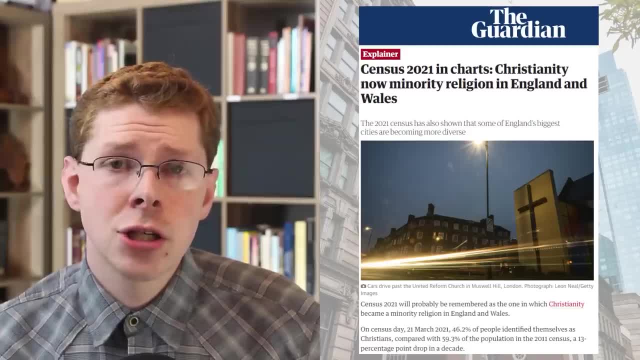 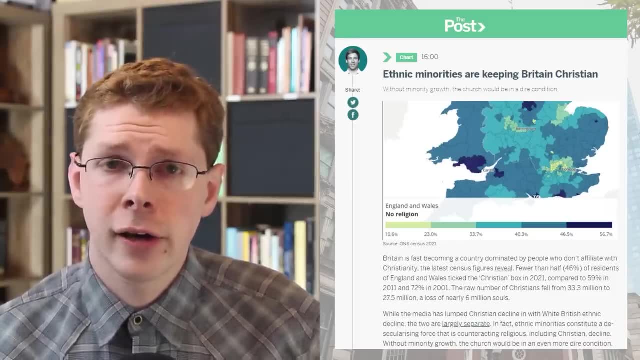 in England and Wales, with only 46.2% claiming it. churches often find their strongest hope to be fervently practicing immigrant populations, which provide new life and new children to declining congregations. The same thing seems likely in the United States, where, from 2010 to 2015,. a majority of immigrants have been Christian. But when talking about the decline of Christianity in America, it's important to note that things are not the same across all Christian traditions. For an extreme example, look at the Amish. In 2000,. there were approximately 178,000. 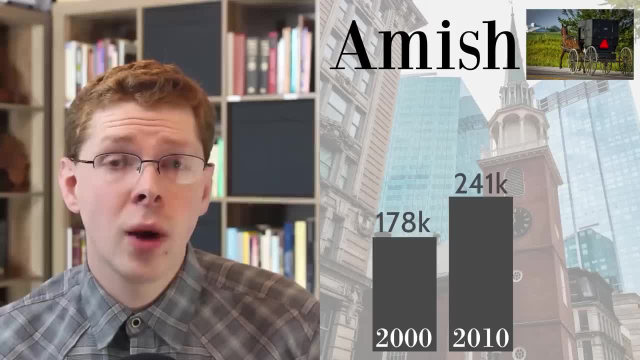 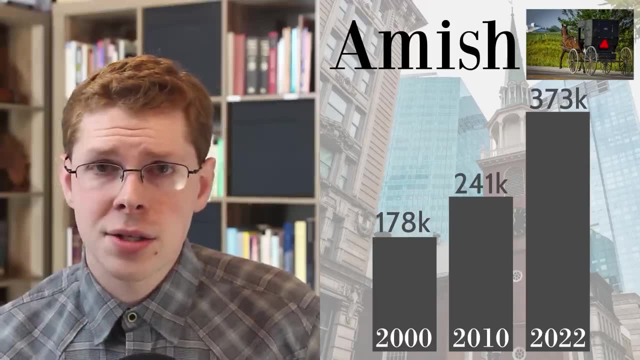 of them. One decade later, in 2010,, the number became 241,000.. In 2022, the estimate was 373,000.. Amish double in number about every 20 years. If that continues, the Amish will begin to pass up. 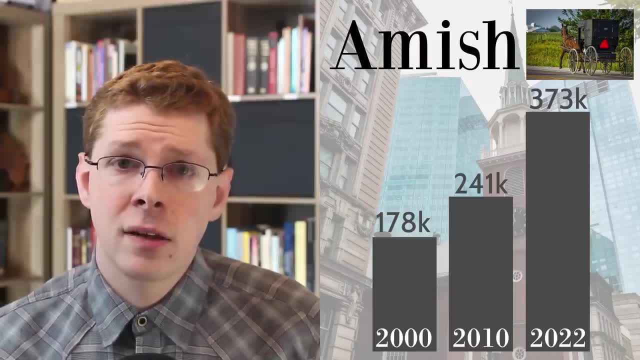 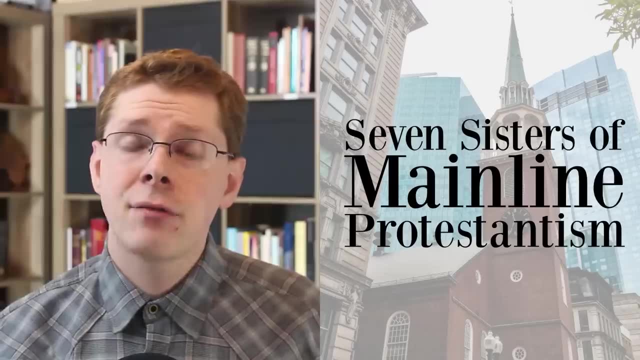 many of these declining mainline denominations very quickly. In fact, they already have been doing so. Another way to look at the mainline is the Seven Sisters, seven mainline denominations that have represented the major traditions in the US. These are the United Methodist Church, Presbyterian. 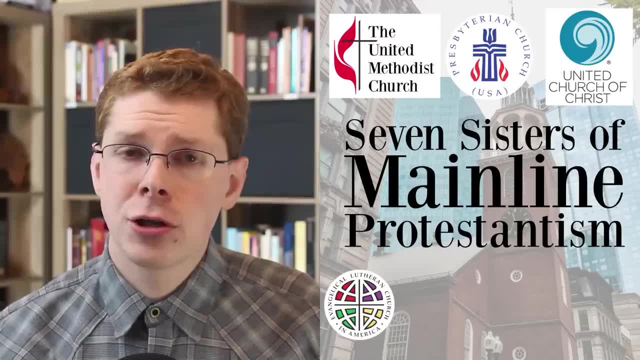 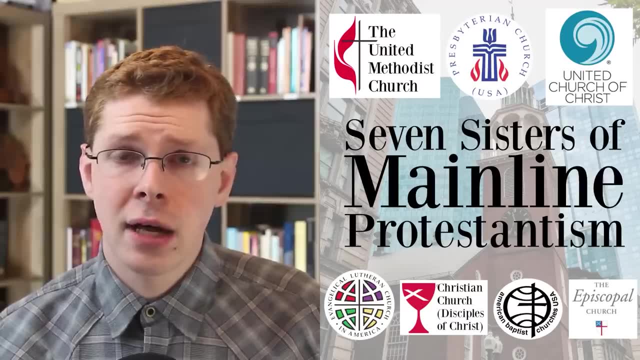 Church USA, United Church of Christ, Evangelical Lutheran Church in America, Christian Church Disciples of Christ, American Baptist Churches USA and the Episcopal Church. And the story is not looking good. American Baptist Churches USA had 1,436,000 members in 2000.. In 2005,, that fell to 1,396,000.. In 2010, 1,308,000.. And in 2015, 1,173,000.. The 2020 number was 1,124,000.. Over two decades. 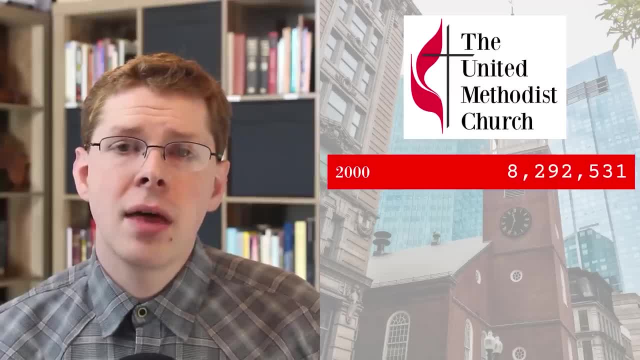 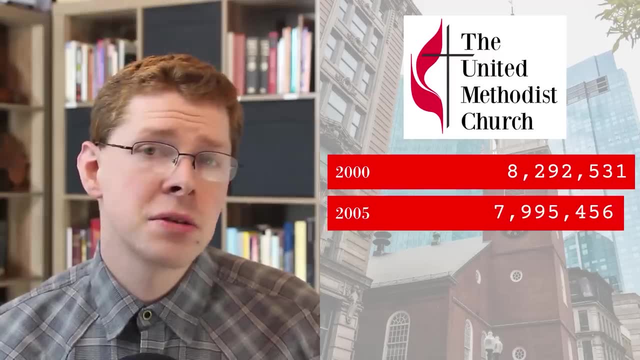 they're down 21.7%. In the year 2000, the United Methodist Church had 8,292,000 US members. It's the largest among the mainline denominations by far. In 2005, that had fallen to 7,995,000. 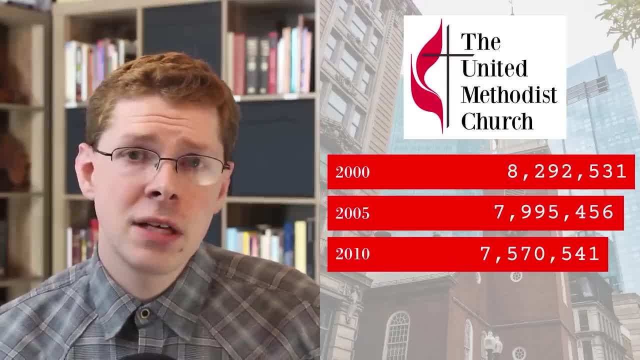 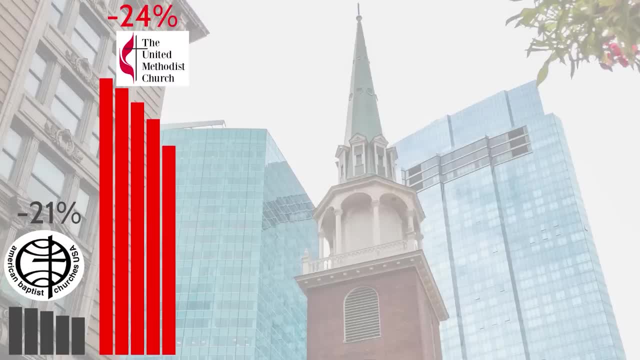 In 2010, 7,570,000.. In 2015, 7,067,000.. And in 2020, 6,268,000.. That's a 24.4% decrease over two decades. There's a lot more ahead you don't want to miss, but I want to let you know what I've. 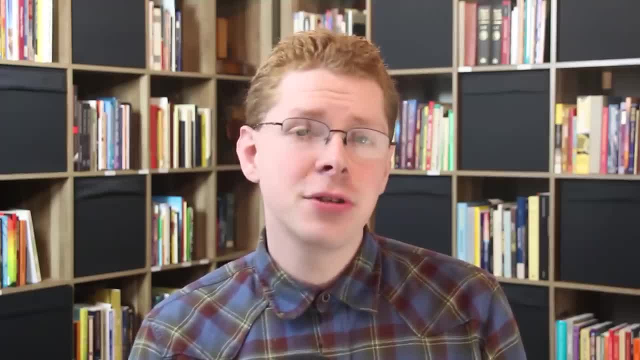 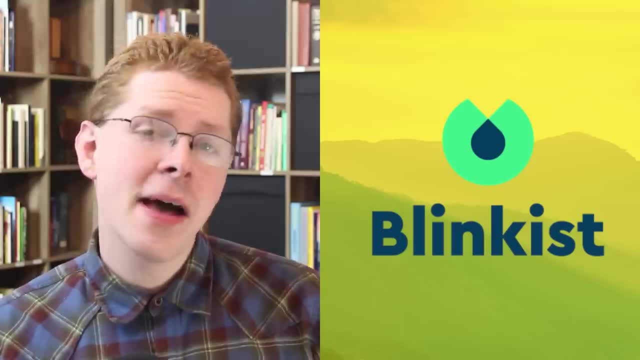 been doing in my car for the last month. I get in and my Bluetooth adapter connects to my phone, and then I start up the Blinkist app to listen to a book in 15 minutes. Normally that means by the time I get to my destination I have another book crossed off my reading. 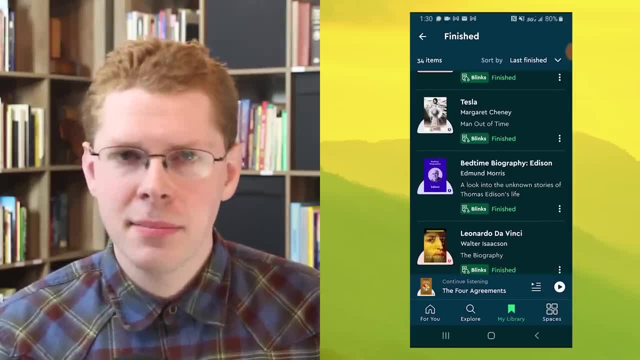 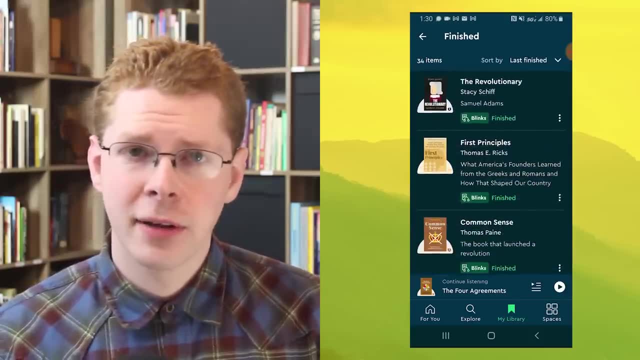 list. Here's a look at my history. I listened to Tesla by Margaret Chaney, a biography about Thomas Edison, one about Leonardo da Vinci, Einstein and Benjamin Franklin. The Gulag Archipelago by Alexander Solzhenitsyn was one that I knew I needed to understand, And 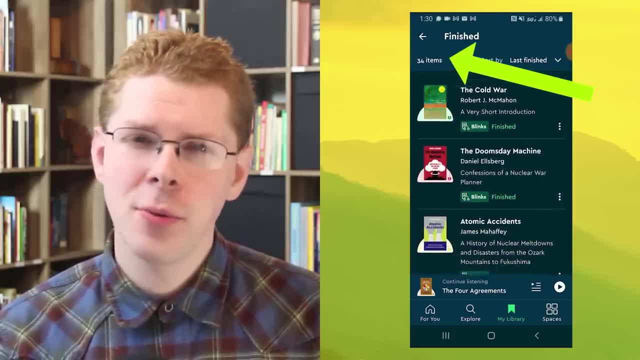 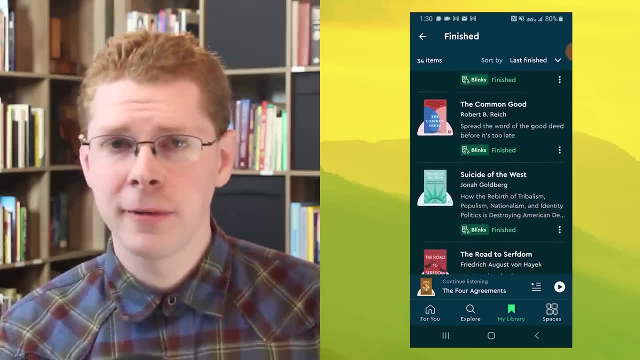 as you can see, I've got 34 Blinks down and there's no way I was going to get these 34 books read without Blinkist. Blinkist helps me use time like driving in the car to learn, And this works because 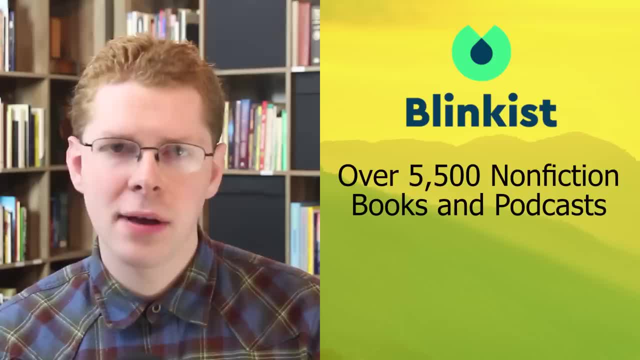 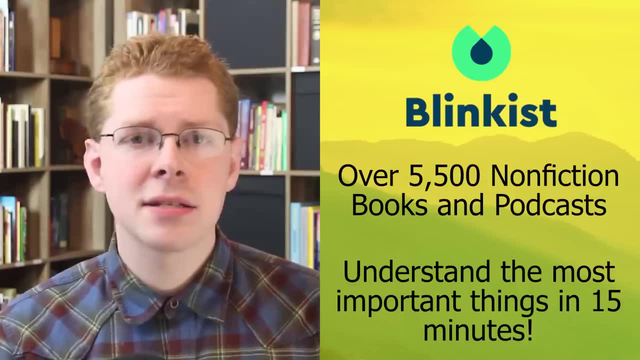 Blinkist allows you to understand the most important things from over 5,500 nonfiction books and podcasts in just 15 minutes. You can read or you can listen. So here's what Blinkist is offering my viewers. Not only can you get 25% off Blinkist Premium. 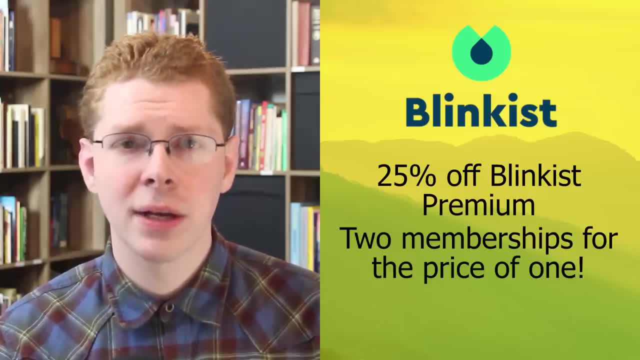 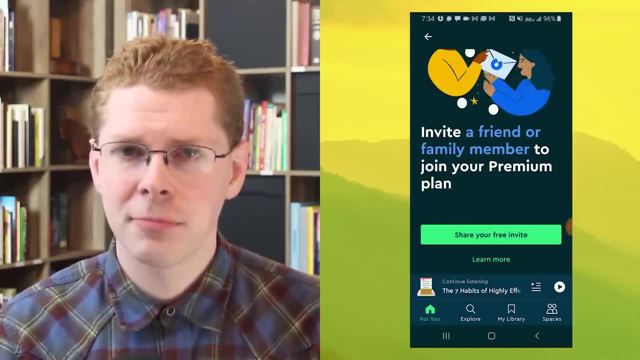 but you can also have effectively two memberships for the price of one with Blinkist's new premium benefit called Blinkist Connect. Anyone with a Blinkist account can share their premium benefits with someone else's free account. Start your 7-day free trial by visiting the link here. It's also in the description And. 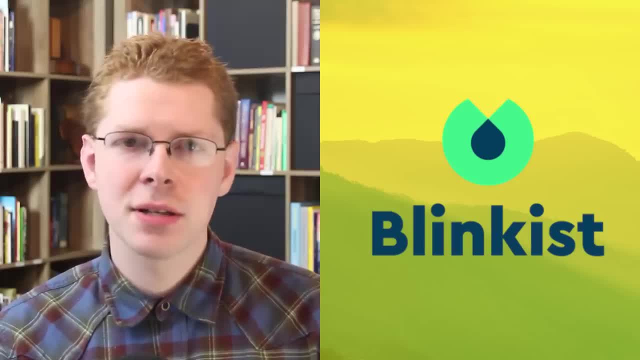 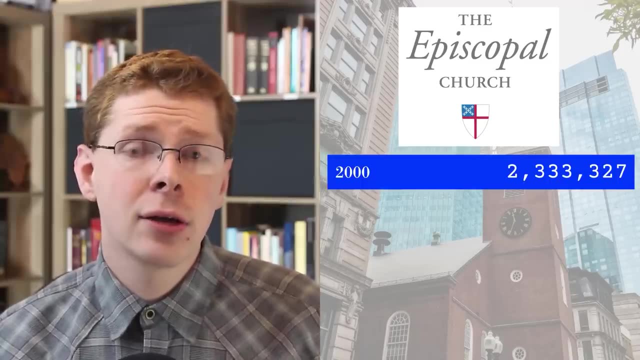 then think of a friend that you want to share with. Thanks to Blinkist for sponsoring this video. Click the link below to subscribe For the Episcopal Church. the numbers began at 2,333,000 at the turn of the century In. 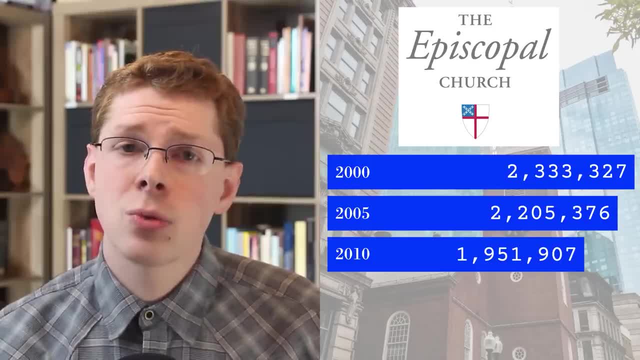 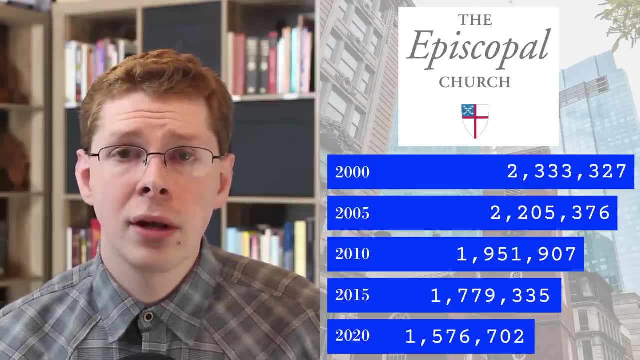 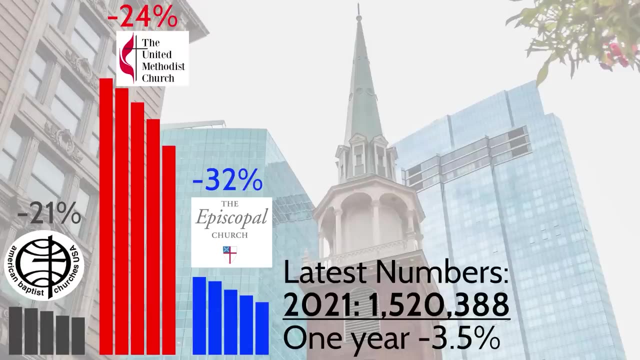 2005, 2,205,000, and then 2010 was 1,951,000.. 2015 brought it to 1,779,000 and 2020, 1,576,000.. That's a 32.42% decline, And in 2021, there was an additional 3.5% decline to 1,520,000. 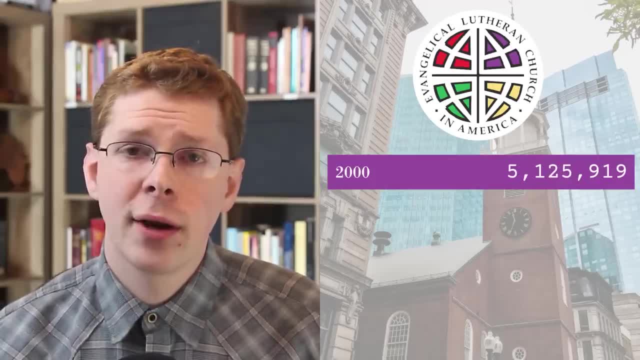 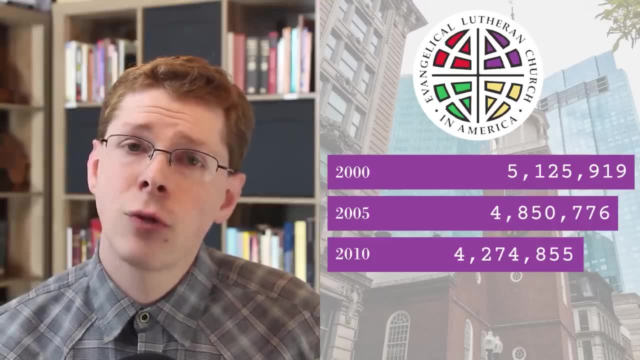 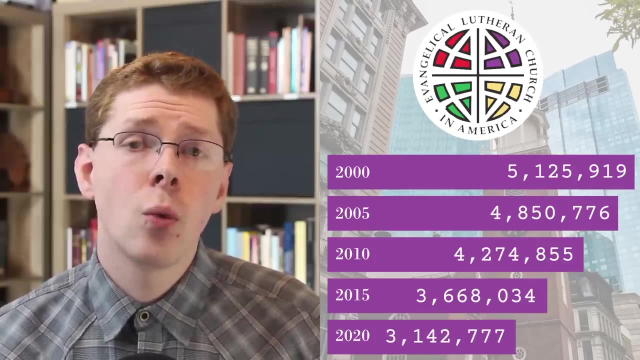 The Evangelical Lutheran Church in America started this millennium with 5,125,000 members. By 2005,, that was shaved down to 4,850,000.. In 2010, it was 4,274,000 and 2015 3,668,000.. The 2020 number was 3,142,000, leaving a 38.6%. 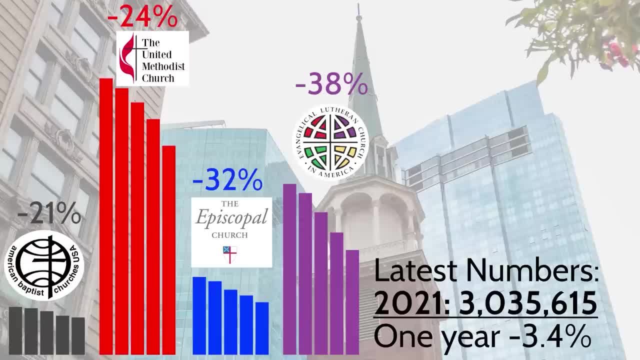 decline since 2000.. There was a further 3.4% decline to 2021's number of 3,035,000.. In the United Church of Christ they had 1,377,000.. The Evangelical Lutheran Church in Africa started this millennium with 5,125,000 members. By 2005, that was shaved down to 4,850,000.. In 2010, it was 4,274,000 and 2015, 3,568,000.. 277,000 members in 2020.. In 2005,, 1,224,000.. In 2010,, 1,058,000.. 2015, 914,000.. And in 2020,. 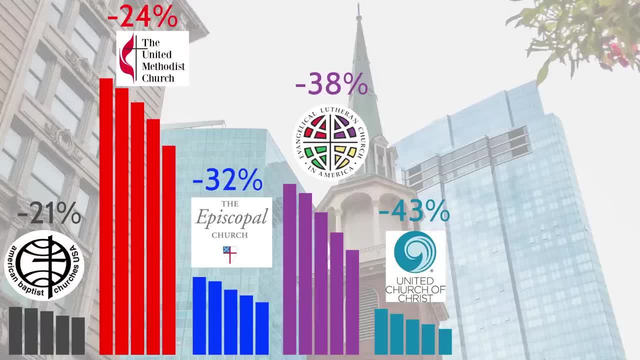 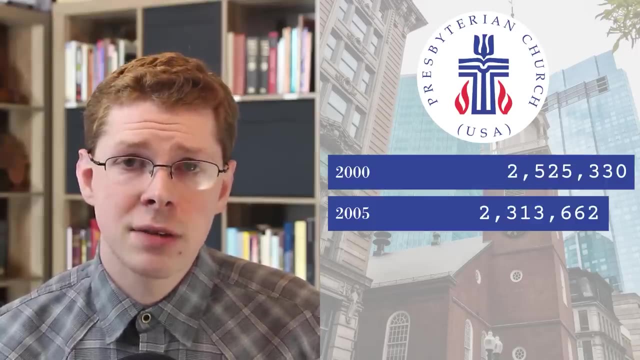 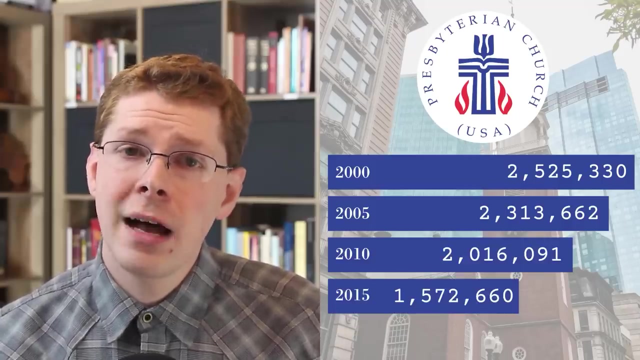 773,000.. Two decades: 43.8% decline. They declined 3.9% in the year following, with the 2021 number being 745,200.. Now the Presbyterian Church USA. In 2000, it had 2,525,000 members. 2005,, 2,313,000.. 2010,: 2,016,000.. 2015,: 1,572,000.. And 2020,. 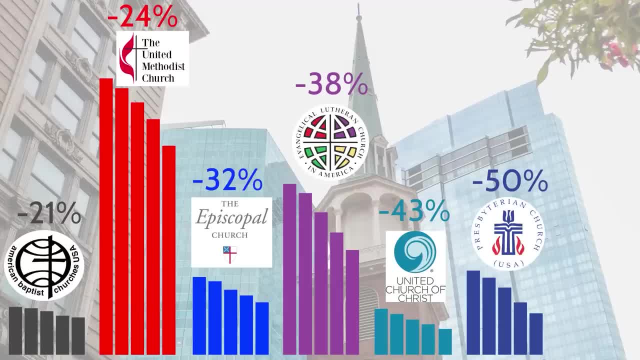 1,245,000.. That's a 50.68% decline since 2000.. The 2021 number drops them to 1,193,000 and over 4% decline in one year. The Christian Church Disciples of Christ was the only one of these. 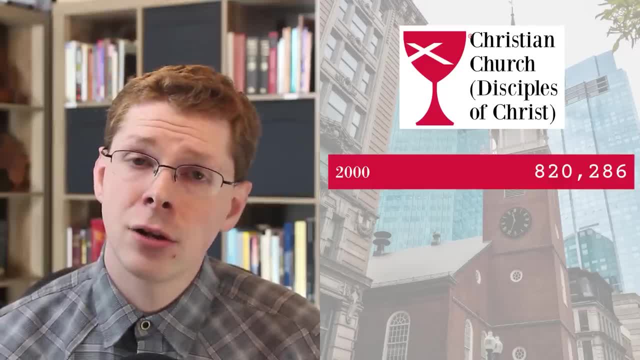 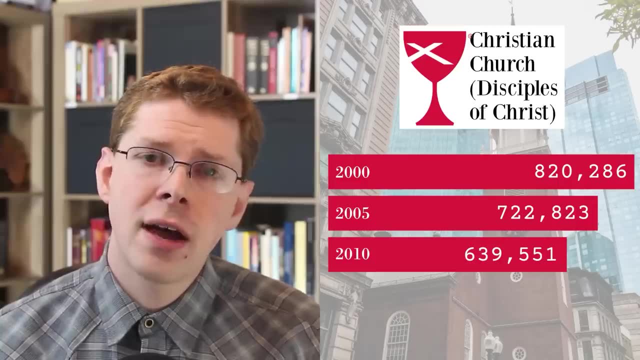 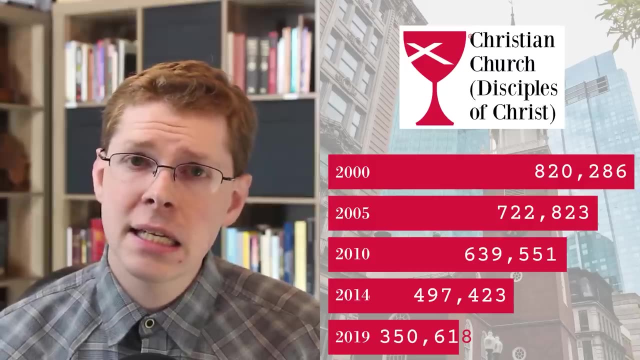 seven sisters to begin the millennium with under a million members at 820,000.. But they could certainly fall further. In 2005, they fell to 722,000.. Then to 639,000 in 2010.. In 2014, the number was 497,000. And the 2019 number was 350,000.. That's only 19. 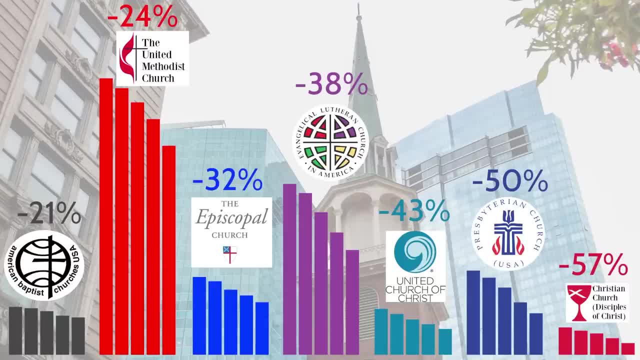 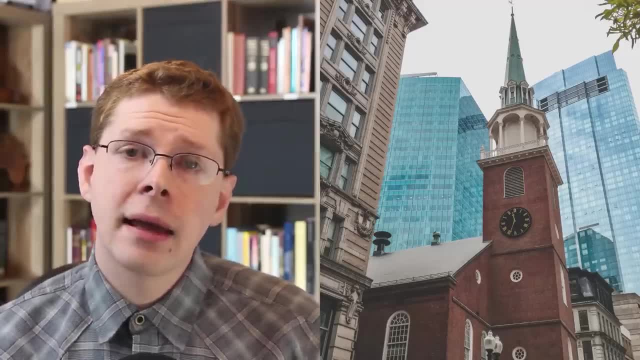 years that I can get the records for as of publication of this video, but it's still a 57.25% decline. There are several reasons for the decline. One of them is simply members dying off. Back in the 2014 Pew Religious Landscape study, mainline Protestants were found to be older as a group than any other major religious tradition. Another reason, though, is members leaving. Pew Research said of that. additionally, more Americans have been leaving mainline Protestantism than joining the tradition. Nearly one in five Americans- 19%- were raised in the. mainline tradition, but more than half of them- 10.4% of all US adults- have left the faith. Mainline Protestants have one of the lowest retention rates of any major religious tradition, with only 45% of those raised in the faith continuing to identify with it as adults. Some members have left mainline churches individually, and sometimes congregations have left one at a time to become independent or join another denomination. However, in several of these mainline denominations, there have been large-scale exoduses within these last 20 years. 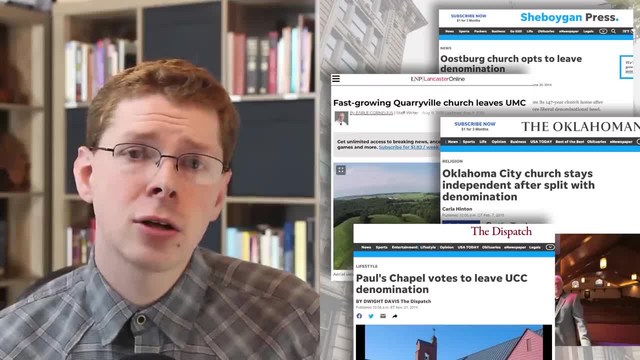 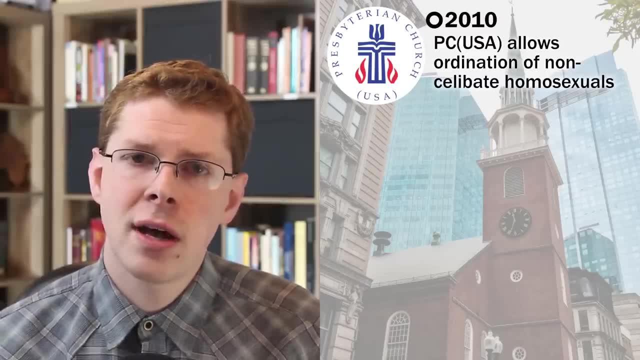 and the main catalyst for the departures have been the ordination of LGBT clergy and same-sex marriage in the mainline denominations. The Presbyterian Church USA allowed the ordination of non-celibate homosexuals in 2010.. As a result, a new denomination, ECO, a covenant order of 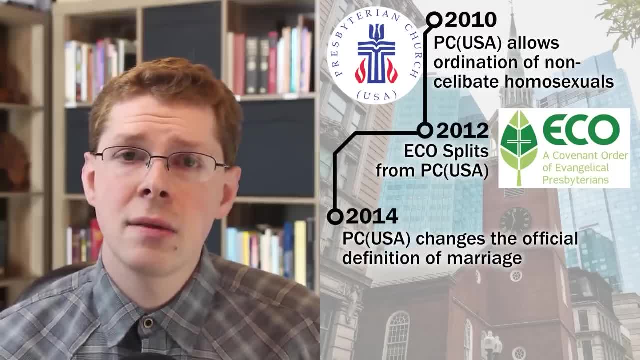 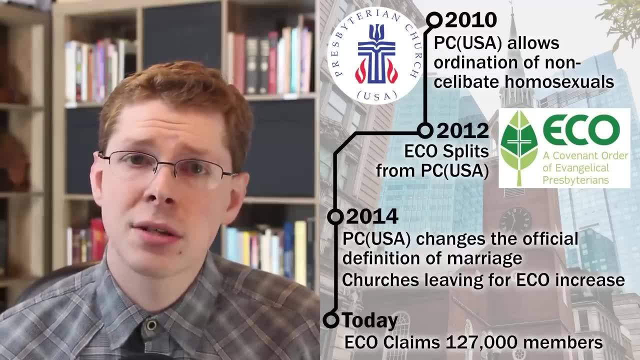 evangelical Presbyterians was formed. The Presbyterian Church USA allowed the ordination of non-celibate homosexuals in 2012.. In 2014,, the PCUSA changed their official definition of marriage and more churches left for ECO. Today, ECO claims 127,000 members, most of which came from former. 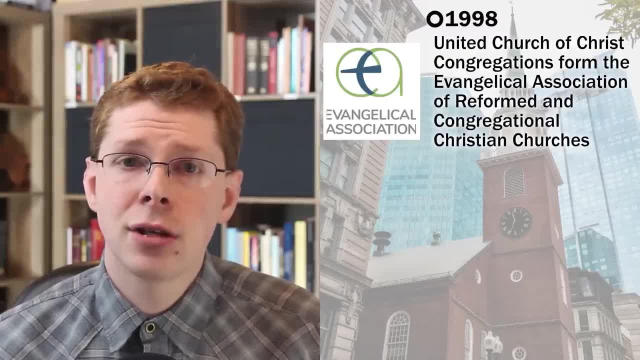 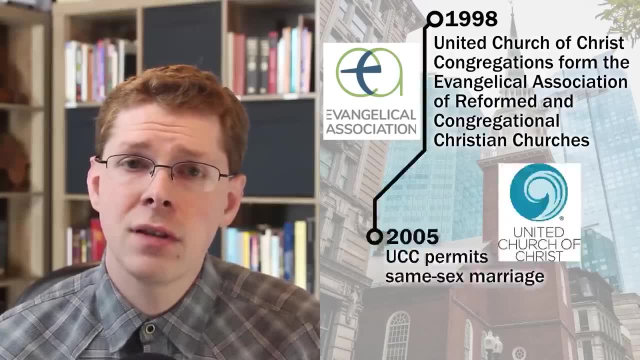 PCUSA congregations. In 1998,, some United Church of Christ congregations formed the Evangelical Association of Reformed and Congregational Christian Churches and when, in 2005,, the UCC began to permit same-sex marriage, many churches left to join it. The Evangelical 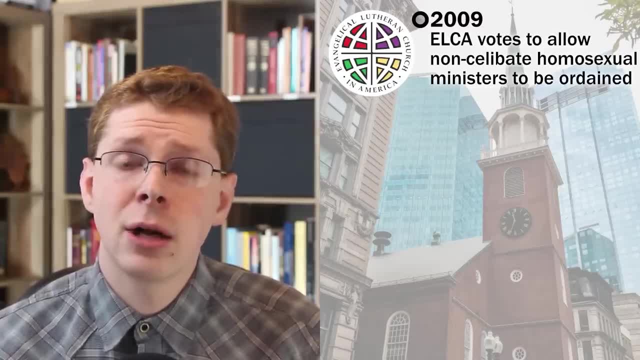 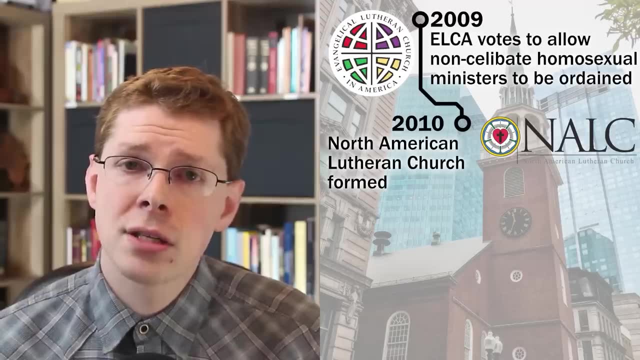 Lutheran Church in America voted to allow non-celibate homosexual members to be able to be ordained in 2009.. In 2010,, the North American Lutheran Church split from the ELCA and has 142,000 members today. Another denomination that took many ELCA churches in the same time frame was 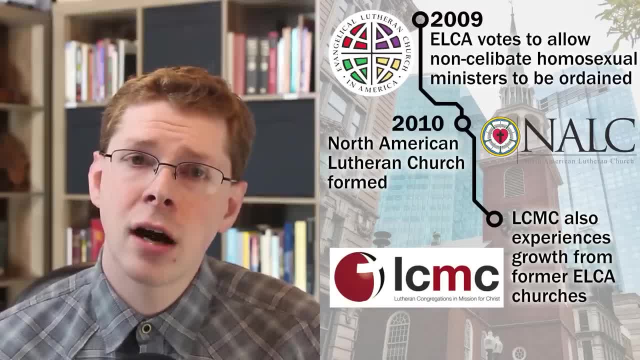 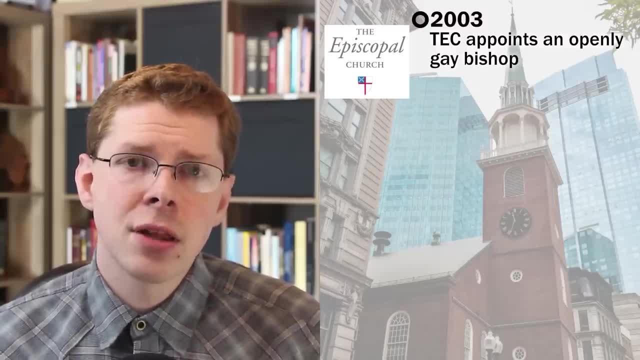 Lutheran Congregations and Mission for Christ, which grew from 210 congregations in 2007 to 960 in 2020.. The Episcopal Church appointed an openly gay bishop in 2003, and late in 2015, the church canons were updated to change their stance on marriage to allow same-sex marriages. Because of 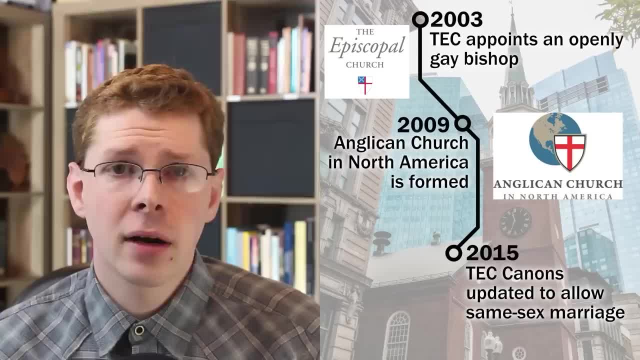 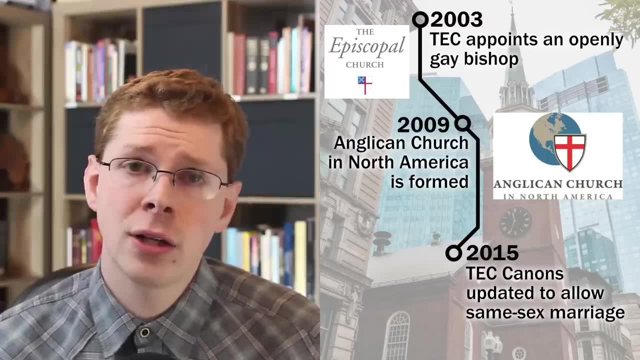 on sexuality. in 2009,, the Anglican Church in North America was formed and grew from 70,000 members in 2011 to 133,000 in 2018, before declining to 122,000 in 2021.. In the American, 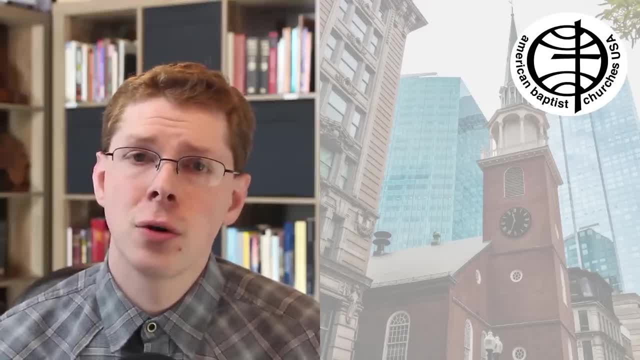 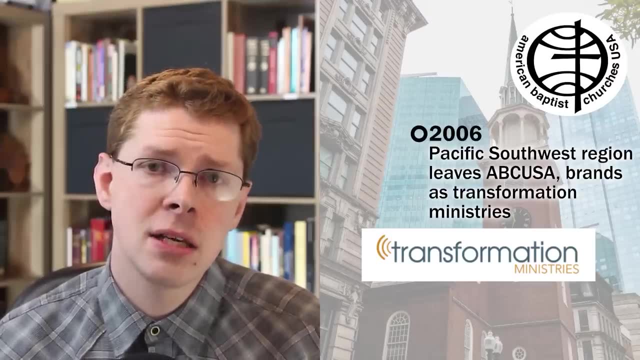 Baptist Churches USA. the Pacific Southwest region of the church as a whole seceded from the denomination in 2006 because the ABC USA allowed members and churches that were affirming of the LGBT movement to remain in the denomination. They have 200 churches and are called Transformation Ministries. First, the United Methodist Church. From the years of 2000 through 2020,, they've seen the second least amount of decline among these seven sisters. but they're quickly going to see those numbers change. As I reported in January 2023, the denomination is splitting and thousands of 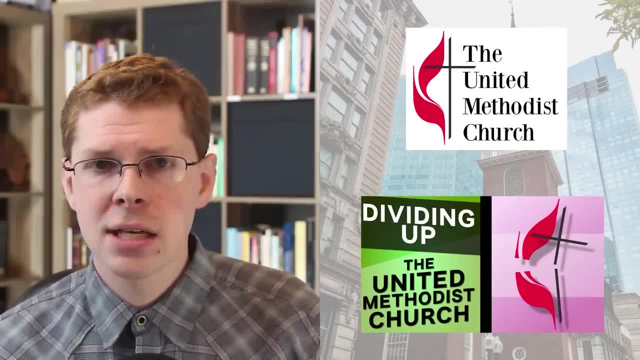 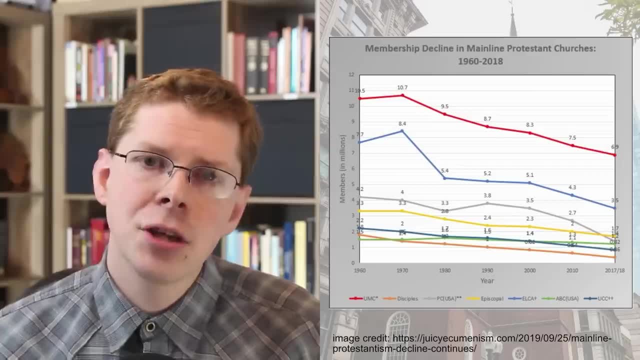 churches are leaving and taking hundreds of thousands of members out of the UMC. With the UMC finally fracturing, this may be the last major split among these seven mainline denominations. LGBT issues did not begin the decline in these denominations, as most have been. declining since the 1960s, but this controversy has hit these churches hard while they're on the way down. So how do mainline churches look as compared to the more conservative denominations in the US? For the evangelical and confessional denominations it's more of a mixed bag. The 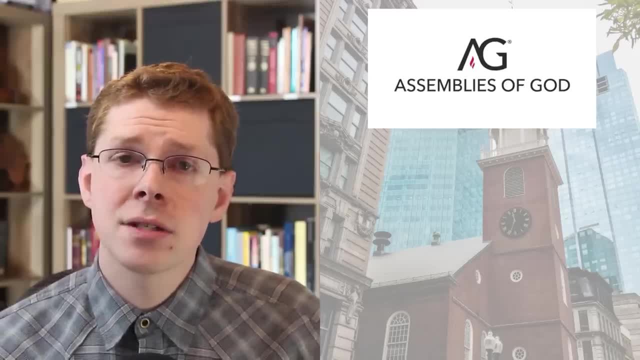 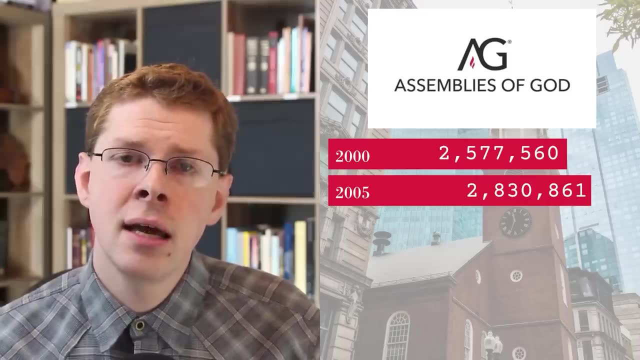 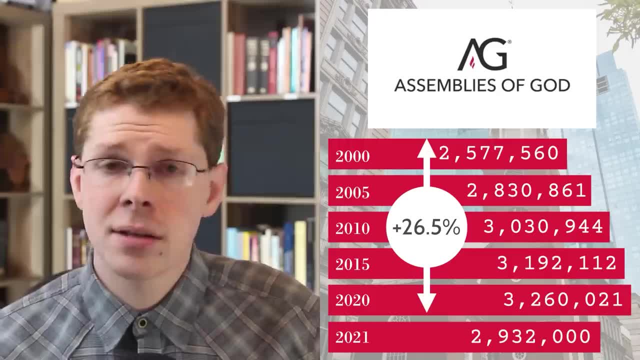 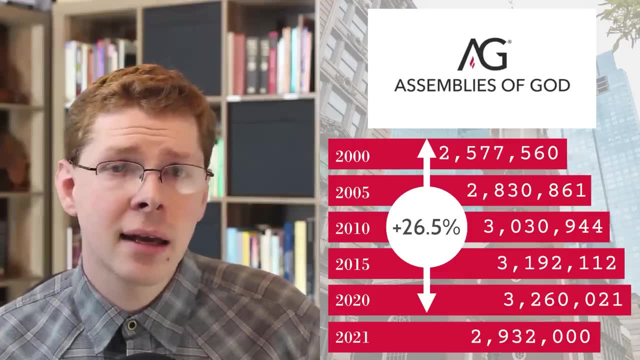 2020 to 2021,. they fell a shocking 10% in one year. COVID-19: a definite factor. They landed at 2,932,000 in 2021, wiping out a decade of growth in one year. The second largest. Presbyterian denomination. the Presbyterian Church in America, which is conservative and confessional, had 306,156 members in 2000,, 331,126 in 2005,, 346,814 in 2010,, 370,332 in 2015, and 383,338 in 2020.. That's a 25% increase over the two decades, But COVID-19 once again. 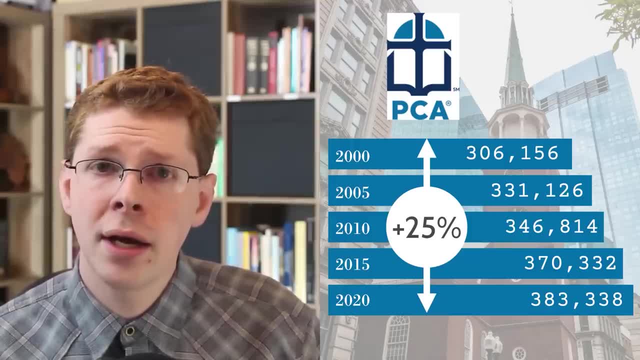 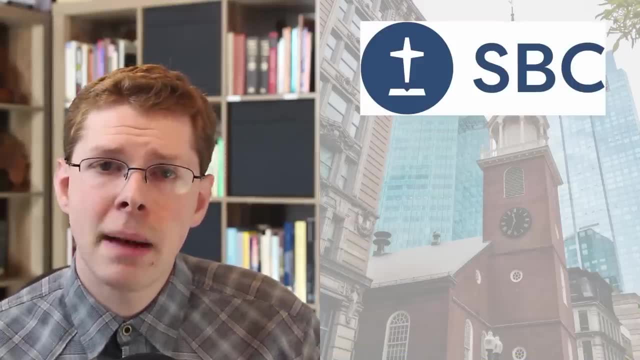 has likely played a part in their decline. From the year of 2020 through 2021, they fell 1.2% to 378,389.. The Southern Baptist Convention is the largest Baptist denomination in the US and it started the. millennium with growth. In 2000, they had 15,960,000 members. They went up to 16,270,000 in 2005.. However, 2006 was their peak and by 2010, they had fallen back to 16,136,000.. By 2015 to 15,294,000, and 2020 to 14,089,000.. The two-decade loss was 11.7%. In 2020, they fell 1.3% to 13,680,000.. The Lutheran Church Missouri Synod is the second largest Lutheran. denomination and is conservative. In 2000,, they had 2,553,000 members. In 2005, 2,440,000.. In 2010, 2,278,000.. In 2015, 2,060,000.. By 2020, they fell under the 2 million mark to 1,861,000, or a 27%. decline since 2000.. In 2020, 2,261,000.. In 2014,: 2,278,000.. In 2015, 2,261,000.. In 2015, 2,261,000.. In 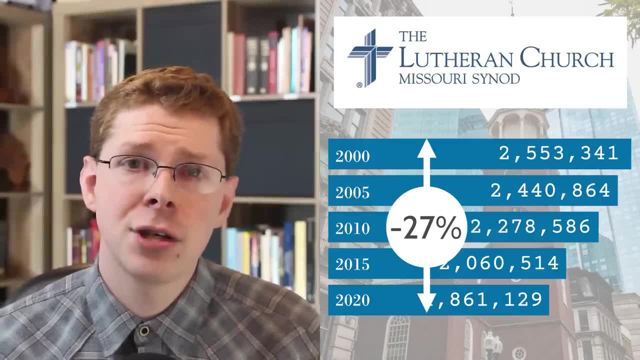 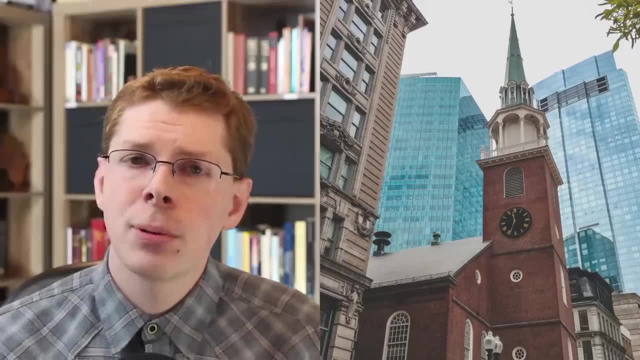 That puts them in the same realm of decline as the mainline denominations. and to top it off, in 2021 they fell a further 2.9% to 1,807,000.. Though precise statistics aren't available, other denominations have seen growth. The Baptist denomination Converge went from 134,000 in 1992 to 194,000 in 2006, to 322,000 in 2020.. The Pentecostal denomination Redeemed Christian Church of God claimed 200 congregations in 2010,, had 720 congregations in 2014, and 921 congregations in 2022. 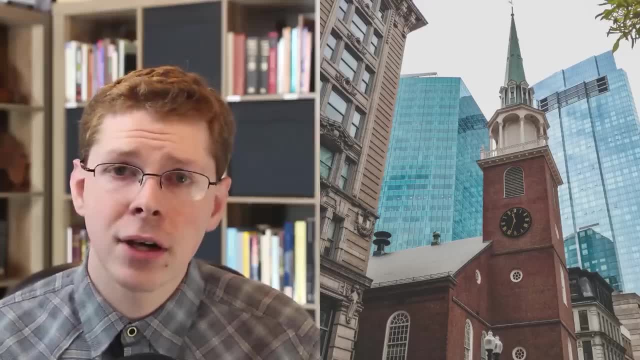 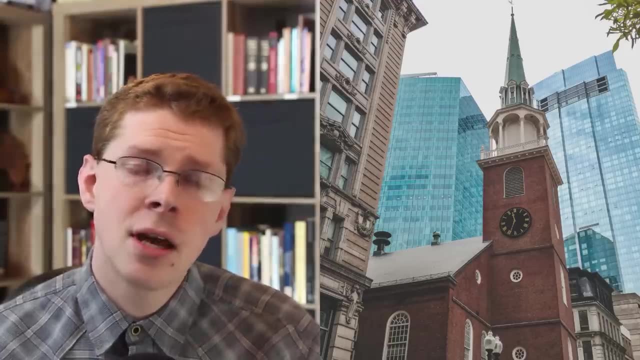 So, although the mainline is declining faster as a whole than many of the conservative denominations, many of these are falling too, But this may be the indication of a trend away from denominations to other church structures. The US Religion Census, which takes place every 10 years, shows that from 2010 through 2020,. 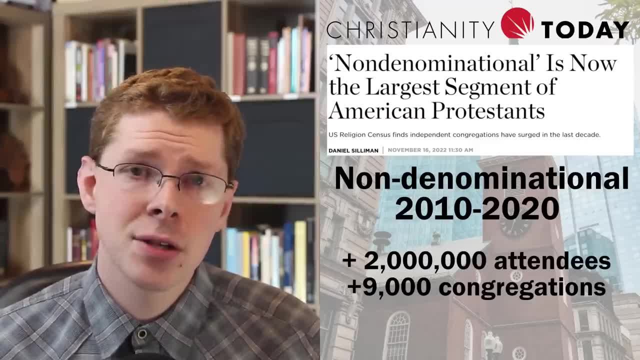 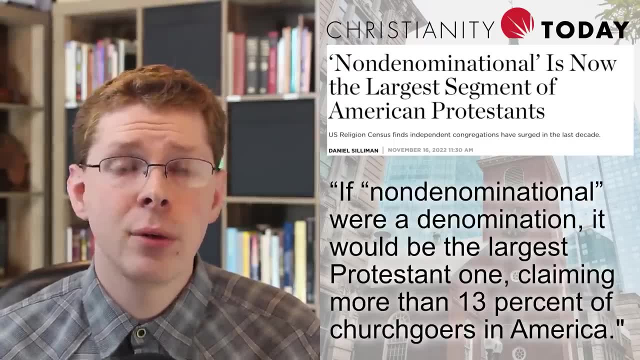 non-denominational churches declined. This grew by 2 million attendees and 9,000 congregations to have 21 million adherents today. Christianity Today reported if non-denominational were a denomination, it would be the largest Protestant one, claiming more than 13% of churchgoers in America. 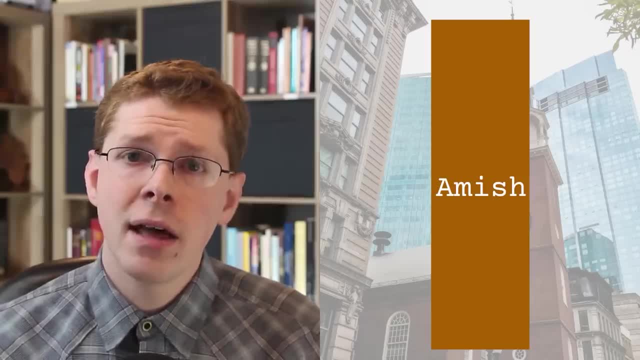 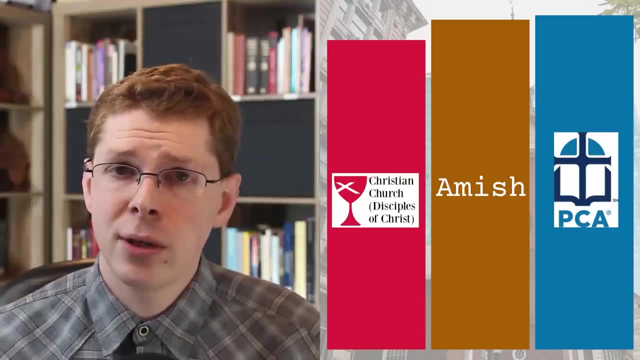 And, as I said, the Amish are becoming more and more of a big deal. They have already surpassed the Christian Church Disciples of Christ, and odds are they will pass the Presbyterian Church in America in membership sometime in 2023, and by the end of the decade they will likely surpass the United Church of Christ. 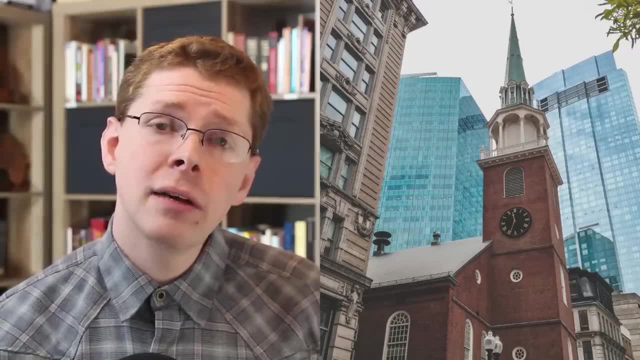 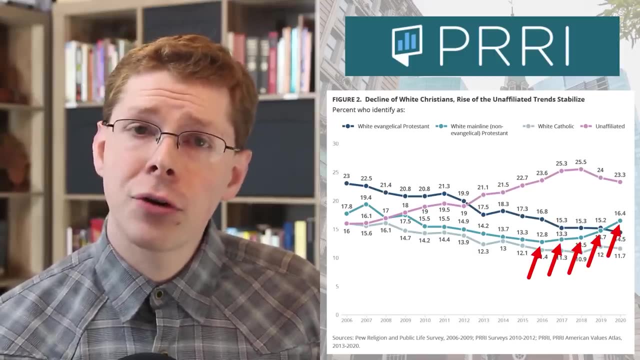 A case of poor service. The survey methodology gave mainline Protestants a short-lived glimmer of hope in 2021, when the Public Religion Research Institute announced that not only had mainline Protestants rapidly grown from 13% to 16% from 2016 to 2020,. 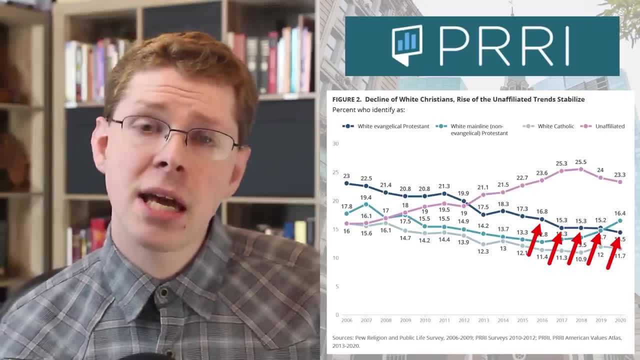 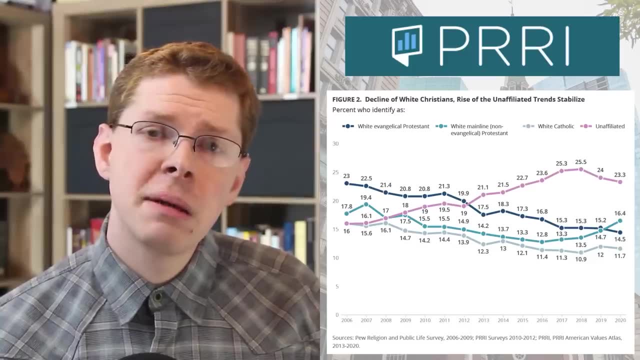 but evangelicals had fallen from 23% to 14% in the same time. A closer look, however, makes us realize that these were mislabeling. The poll didn't ask anything about what denominations people were a part of, but rather made assumptions based on their beliefs. 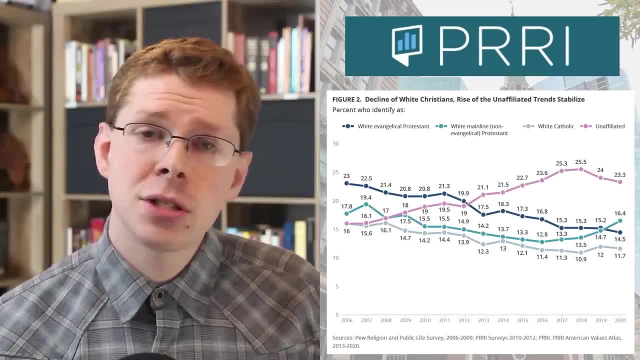 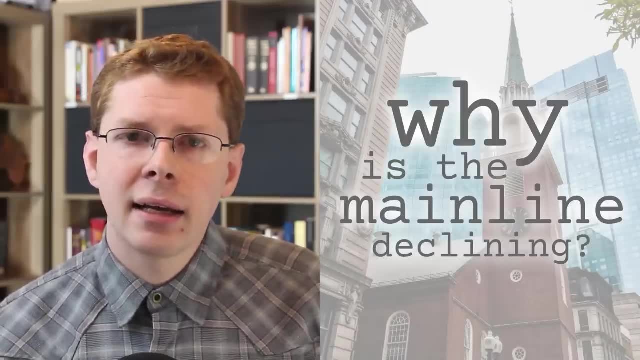 What the data did show, however, was that while the mainline denominations are growing, some of their beliefs are now taking hold even within evangelical denominations. Why is the mainline declining? Let's look at a few responses from differing views. 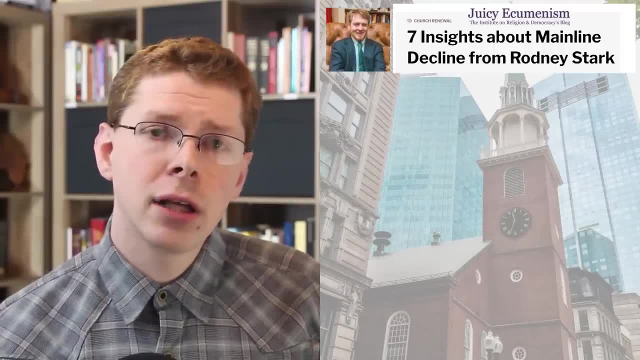 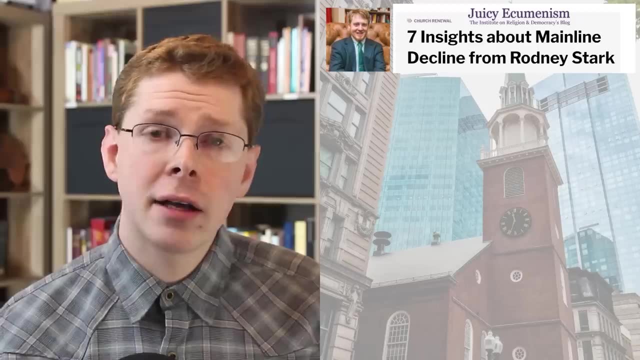 On the conservative side. Joseph Rossell, a writer for the Institute on Religion and Democracy, mined seven concise statements about the state of mainline Protestantism from the book The Triumph of Faith by Rodney Stark. Here they are. Number one: Protestantism is as strong as ever in America. 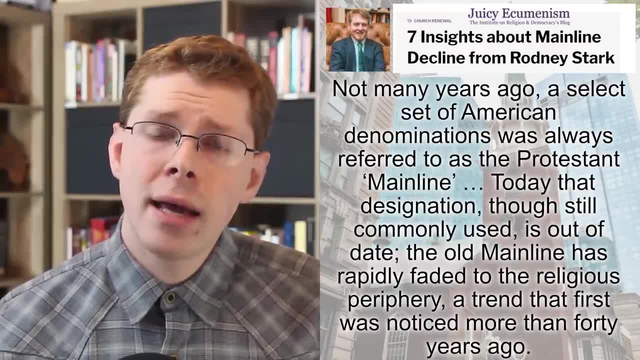 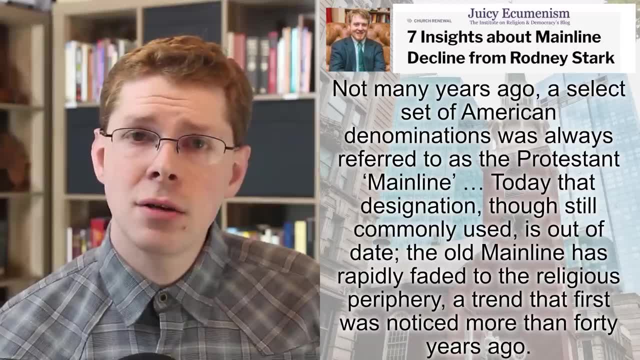 Only the names have changed. Number two: not many years ago, a select set of American denominations. Number two: not many years ago, a select set of American denominations was always referred to as the Protestant mainline. Today, that designation, though still commonly used, is out of date. 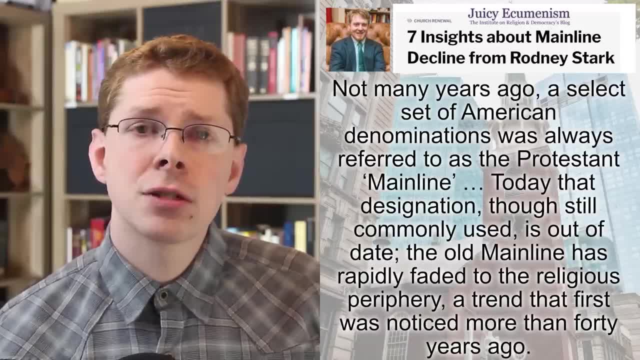 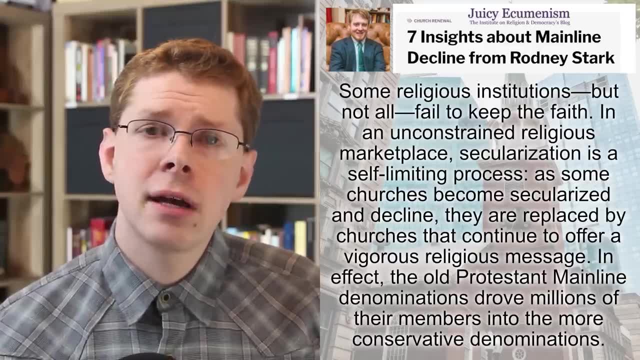 The old mainline has rapidly faded to the religious periphery, a trend that first was noticed more than 40 years ago. Number three: some religious institutions, but not all, failed to keep the faith In an unconstrained religious marketplace. secularization is a self-limiting process. 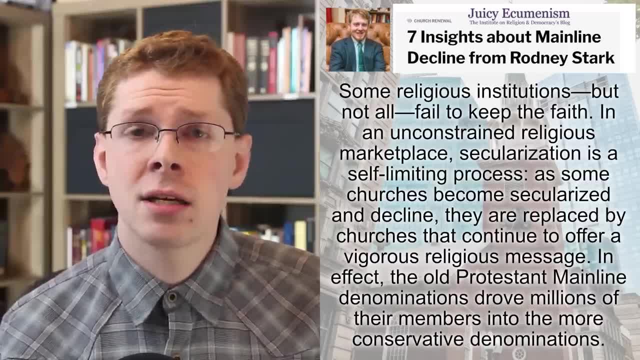 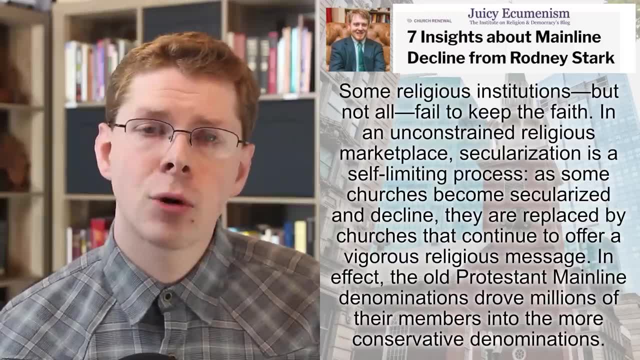 As some churches become secularized and decline, they are replaced by churches that continue to offer a vigorous religious message. The old Protestant mainline denominations drove millions of their members into the more conservative denominations Number four: the wreckage of the former mainline denominations is strewn upon the shoal of a modernist theology. 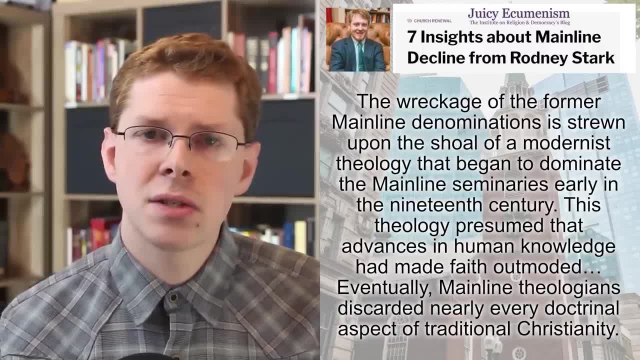 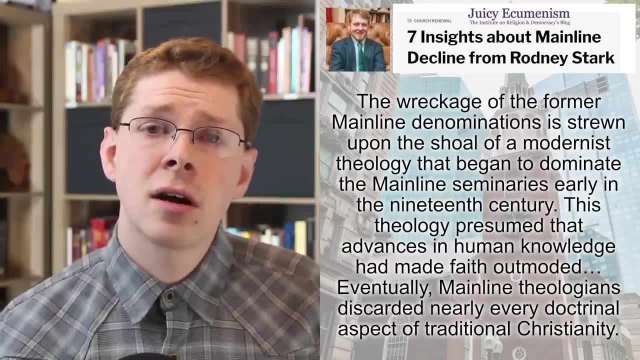 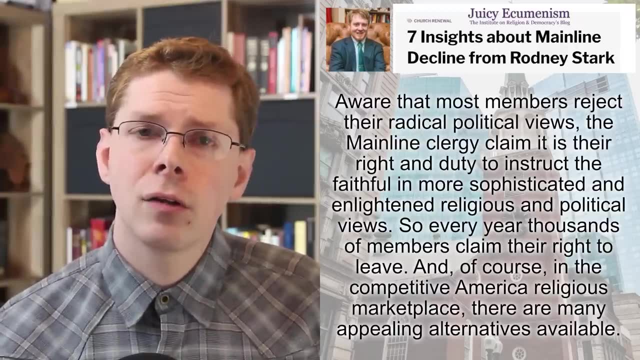 that began to dominate the mainline seminaries early in the 19th century. This theology presumed that advances in human knowledge had made faith outmoded. Eventually, mainline theologians discarded nearly every doctrinal aspect of traditional Christianity. Number five, aware that most members reject their radical political views, 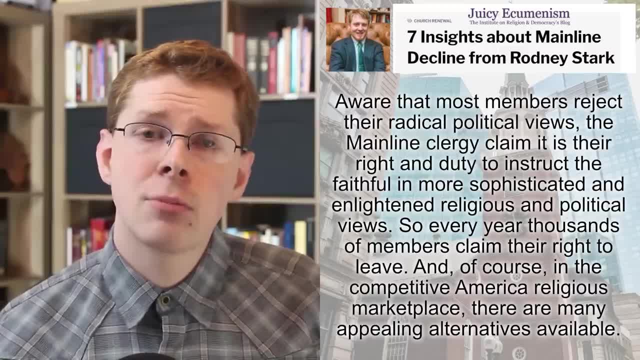 Number five: aware that most members reject their radical political views, claim it is their right and duty to instruct the faithful in more sophisticated and enlightened religious and political views. claim it is their right and duty to instruct the faithful in more sophisticated and enlightened religious and political views. 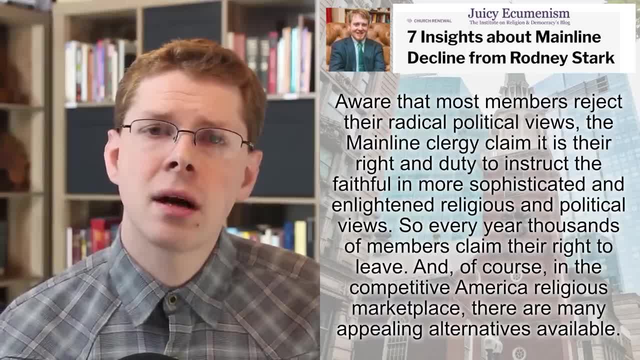 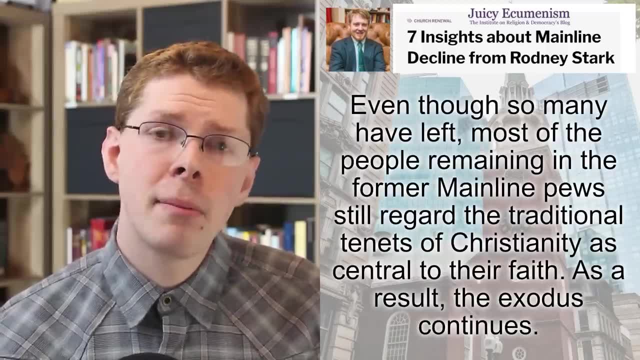 So every year thousands of members claim their right to leave And of course, in the competitive American religious marketplace there are many appealing alternatives available. Number six: even though so many have left, most of the people remaining in the former mainline pews. 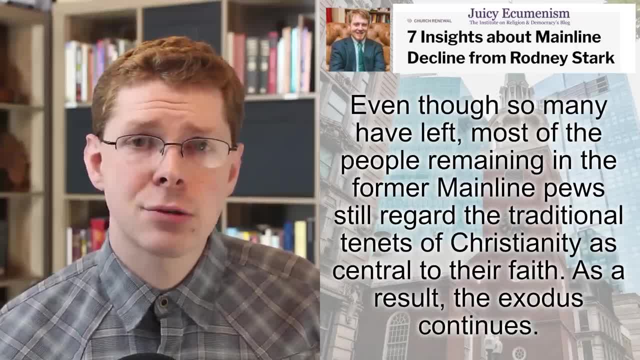 still regard the traditional tenets of Christianity as central to their faith. As a result, the exodus continues. Number seven: many liberals have attempted to make a virtue of the mainline decline. Number seven: many liberals have attempted to make a virtue of the mainline decline. 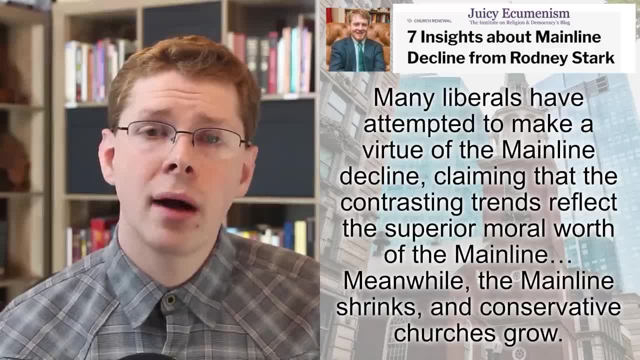 and yet even the latest interesting trends reflect the superior moral worth of the mainline. Meanwhile, the mainline shrinks and conservative churches grow Deanárias difference. Vocês achouem Éper querem Andao H? quién é que stable e conv clubs? 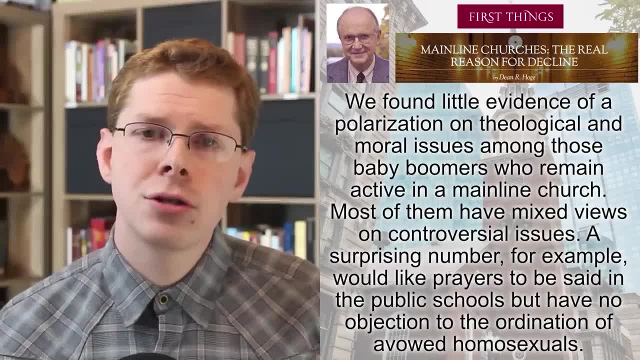 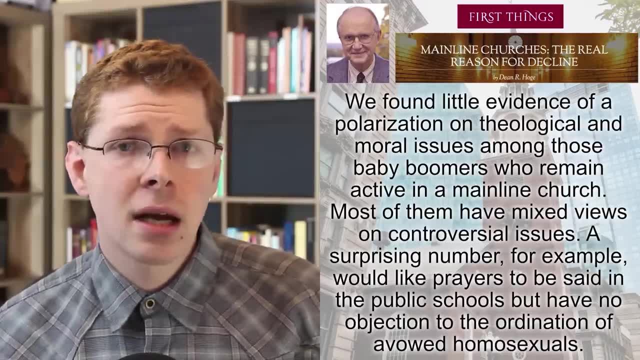 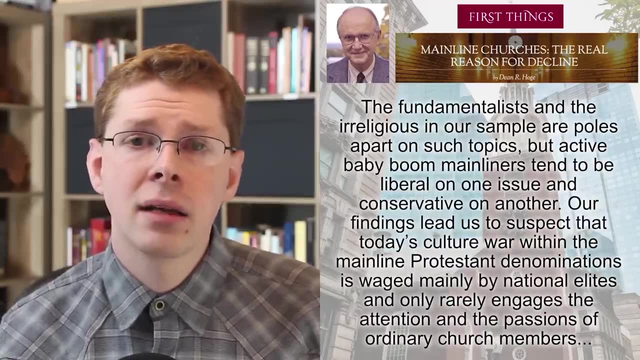 who suffered from a political crisis vis à vis achieve was given the cover of some minuscule incident. we found little evidence of a polarization of theological and moral issues among a minority who had顯 azam thanks of yeux. Most of them have mixed views in a mainline church. 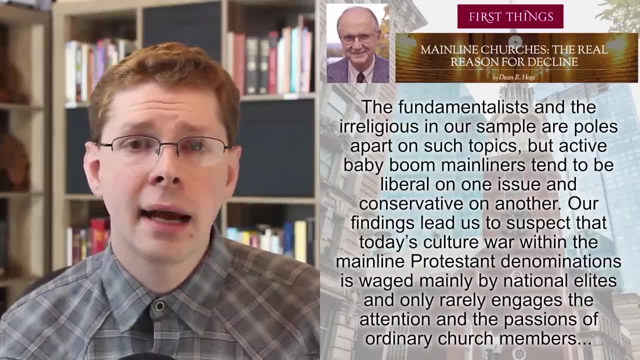 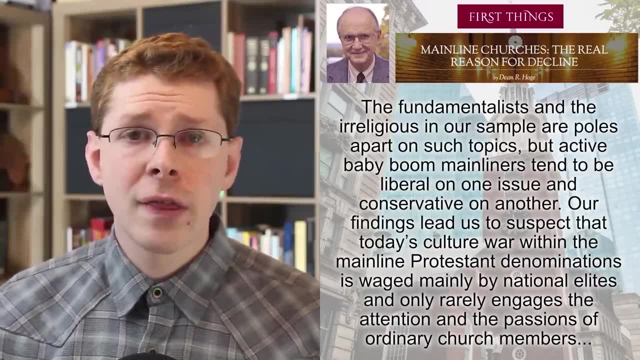 the irreligious in our sample are poles apart on such topics, but active baby boon mainliners tend to be liberal on one issue and conservative on another. Our findings lead us to suspect that today's culture war within the mainline Protestant denominations is waged mainly by national elites. 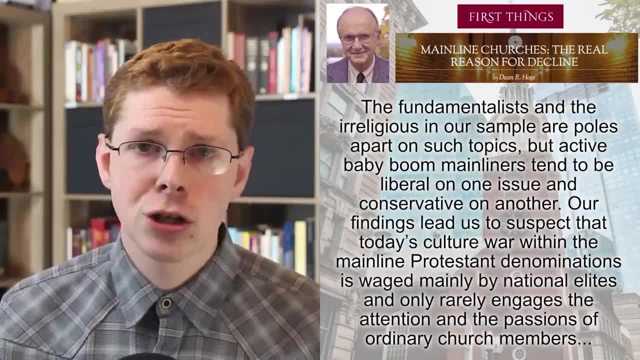 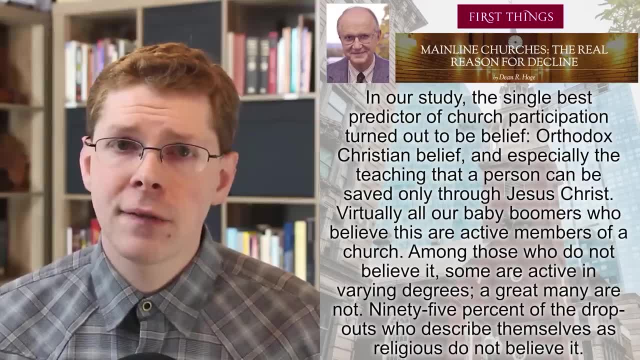 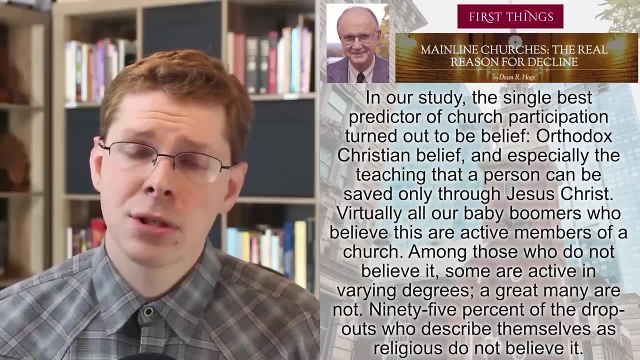 and only rarely engages the attention and the passions of ordinary church members. In our study, the single best predictor of church participation turned out to be belief, Orthodox Christian belief, and especially the teachings that a person can be saved only through Jesus Christ. Virtually all our baby boomers who believe this are active members of a church. Among those who 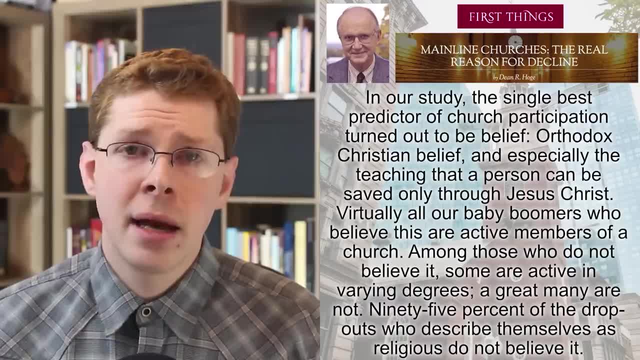 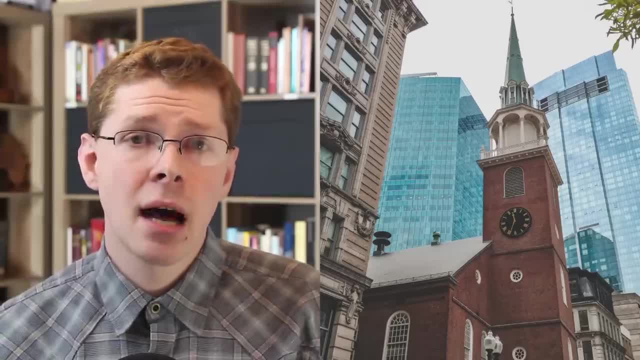 do not believe it. some are active in varying degrees. a great many are not. 95% of the dropouts who describe themselves as religious do not believe it. Another explanation given by some is that this is just the way it always happens: New upstarts push out the old mainline People, like something. 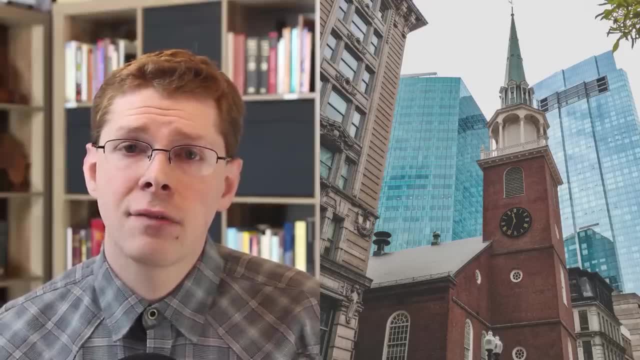 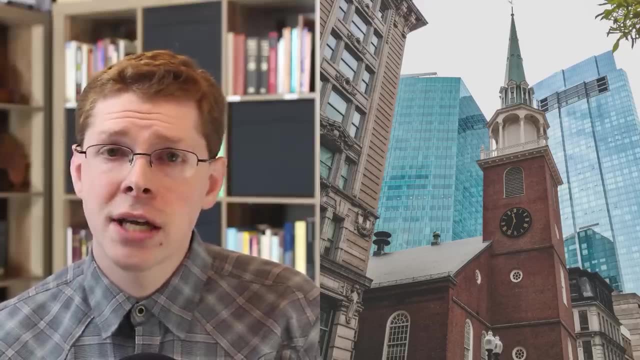 fresh. The mainline is going down, and now we're seeing the beginning of the decline for the following generation of denominations too. like the Southern Baptist Convention, The non-denominational churches, megachurches and multi-site churches are the new flashy alternative. But one day. 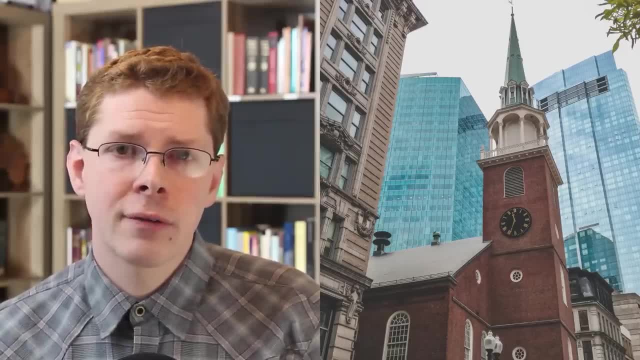 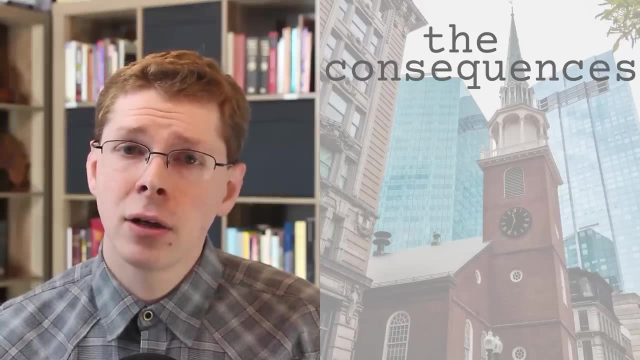 they themselves will become the mainline and they will be pushed out for whatever the next thing is. So what will the consequences of mainline decline be? When congregations in these denominations get small enough, they need to look at either closing down or at a merger, Merging two small congregations. 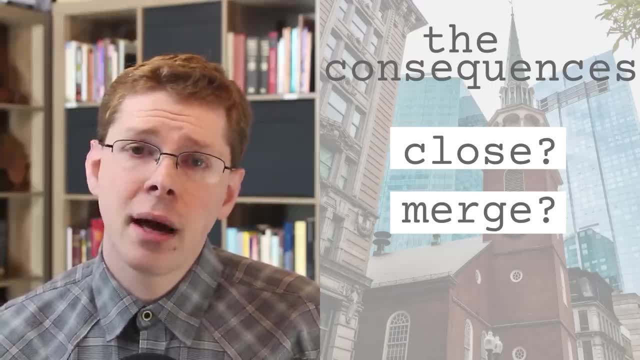 together can keep them alive a bit longer, halving the costs of building, upkeep and perhaps giving a new feeling of life to a congregation. It's possible that this could extend beyond just the local level to the mainline, But we don't know for sure. We don't know for sure. We don't know. 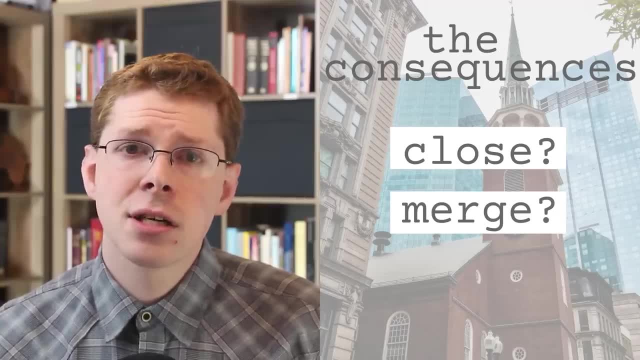 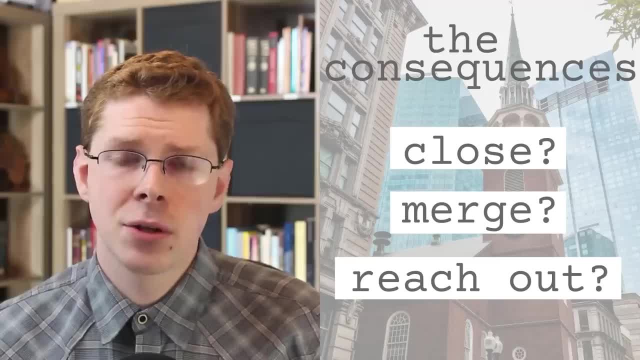 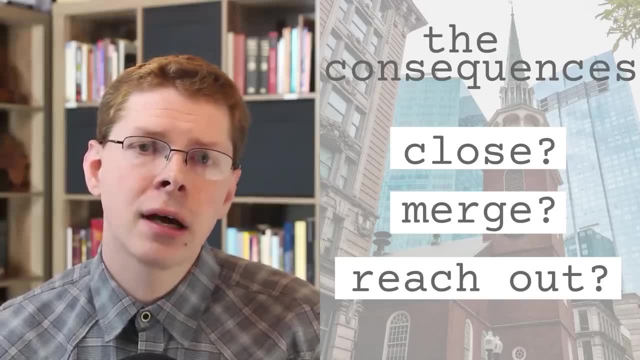 churches in these denominations will do whatever they can to get young families in the doors. New outreaches to younger people in the end are the only way they could see a real turnaround. But it's hard to get young people to come if the inside of the church looks like a seniors night. 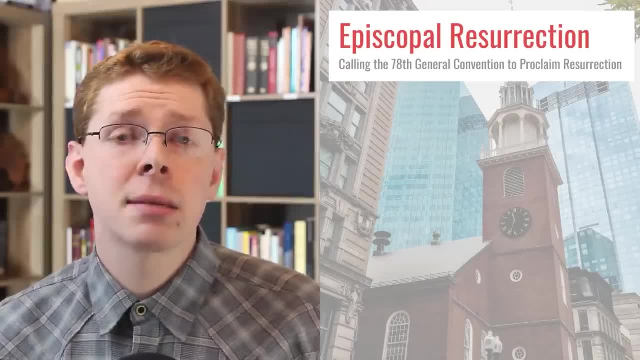 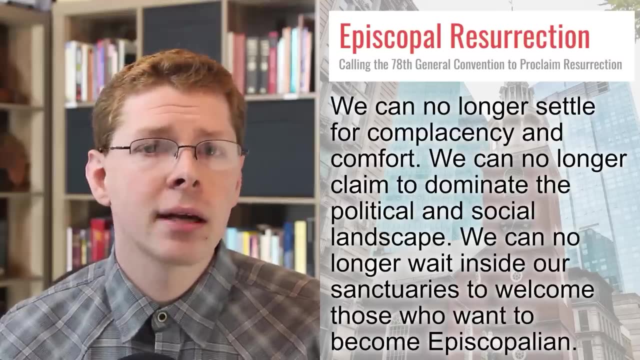 A group called Episcopal Resurrection in 2015 recognized the problem, saying: We can no longer settle for complacency and comfort. We can no longer claim to dominate the political and social landscape. We can no longer wait inside our sanctuaries to welcome those who 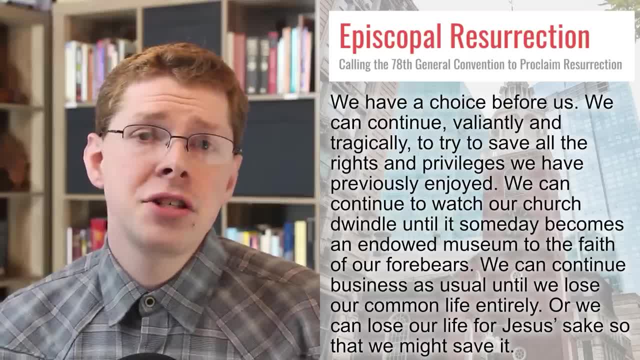 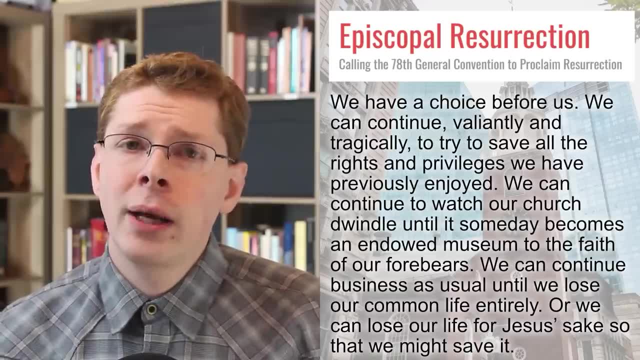 want to become Episcopalian. We have a choice before us. We can continue, valiantly and tragically, to try and save all the rights and privileges we have previously enjoyed. We can continue to watch our church dwindle until it someday becomes an endowed museum to the faith of our forebearers. 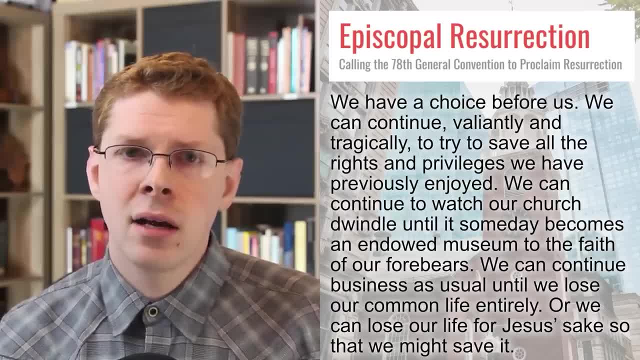 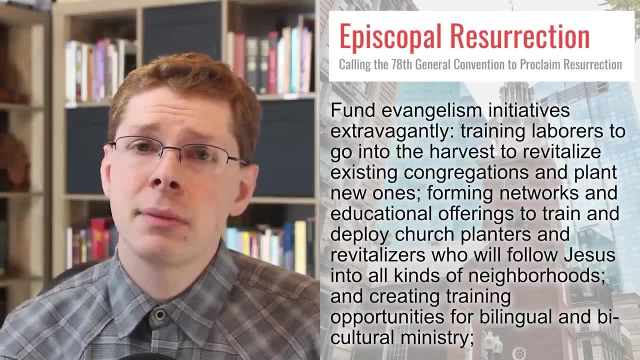 We can continue business as usual until we lose our common life entirely, Or we can lose our life for Jesus' sake, so that we might be able to live a better life. We can continue to live a better life. Some of the solutions they suggested were: fund evangelism initiatives extravagantly. 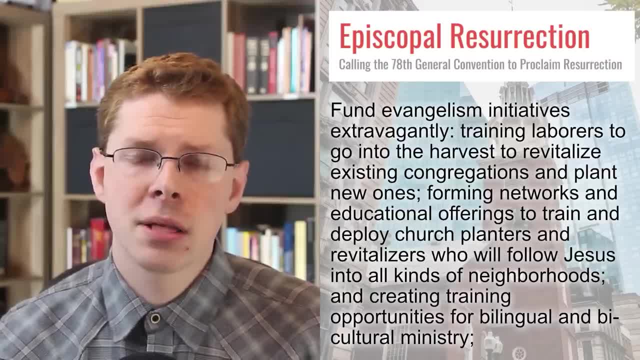 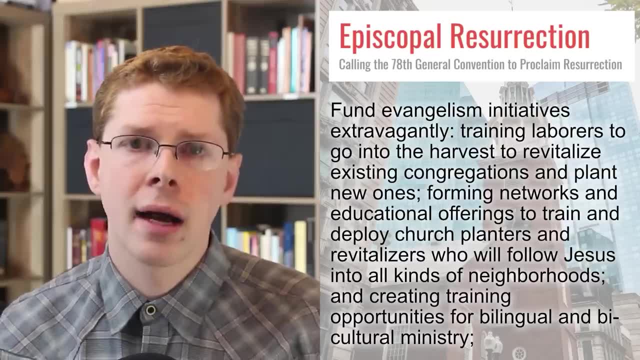 training laborers to go into the harvest to revitalize existing congregations and plant new ones. forming networks and educational offerings to train and deploy church planners and revitalizers who will follow Jesus into all kinds of neighborhoods. and creating training opportunities for bilingual and bicultural ministry. Release our hold on buildings. 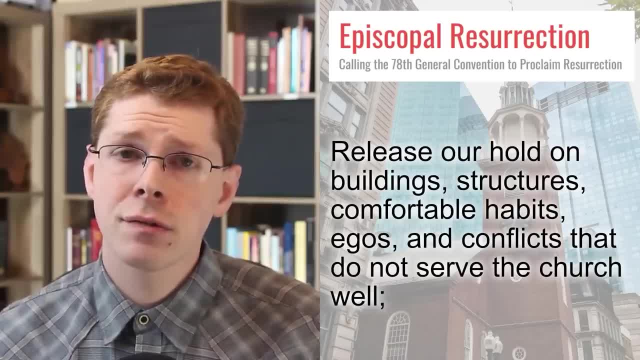 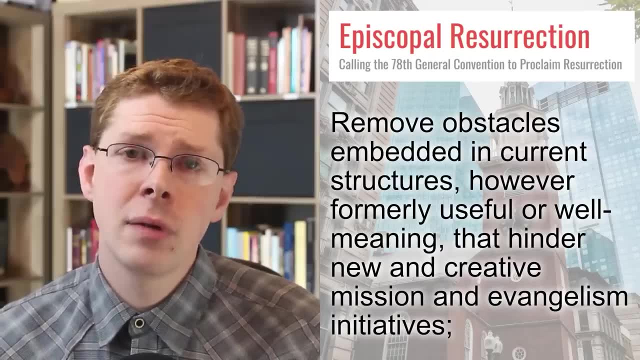 structures, comfortable habits, egos and conflicts that do not serve the church well. Remove obstacles embedded in current structures, however formally useful or well-meaning, that hinder new and creative mission and evangelism initiatives. Refocus our energies from building up a large, centralized, expensive, hierarchical 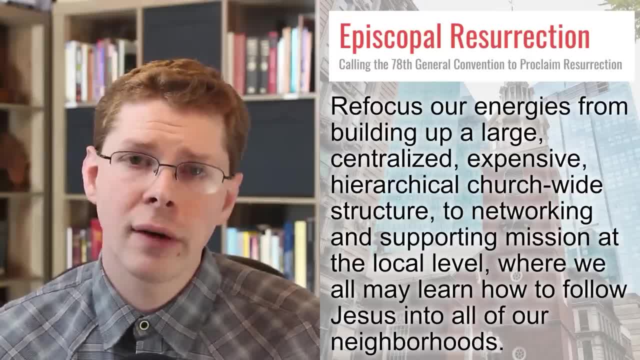 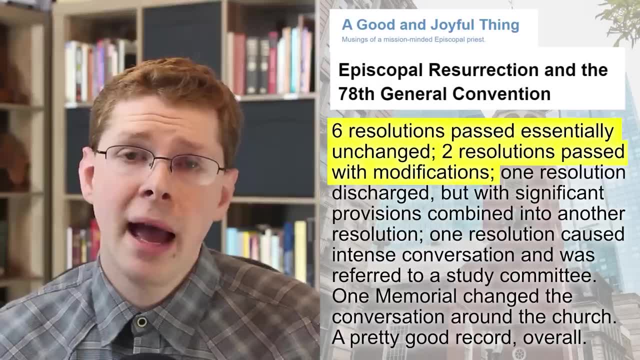 church-wide structure to networking and supporting mission at the local level, where we all may learn how to follow Jesus into all of our neighborhoods. As a result of their efforts, many proposed resolutions were passed at the General Convention in 2015.. The goal: To avoid predictions like the